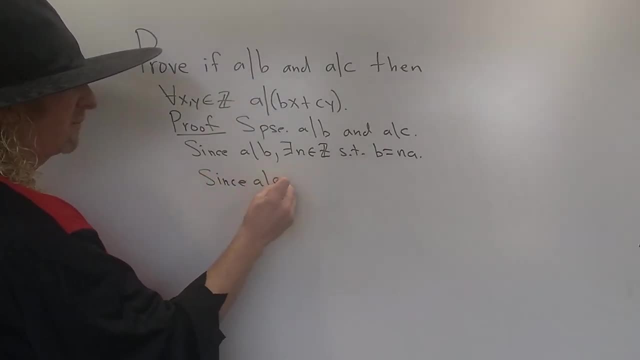 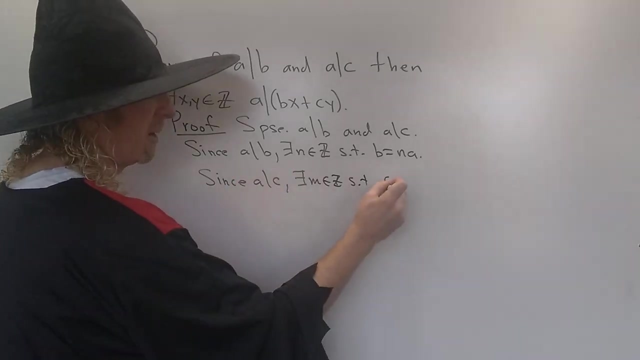 Likewise, since a divides c, this means there exists an integer n. we have to use a different letter, such that c is a multiple of a, so c is equal to ma. Good stuff, Okay. so all we've done so far is write down our assumption, right? 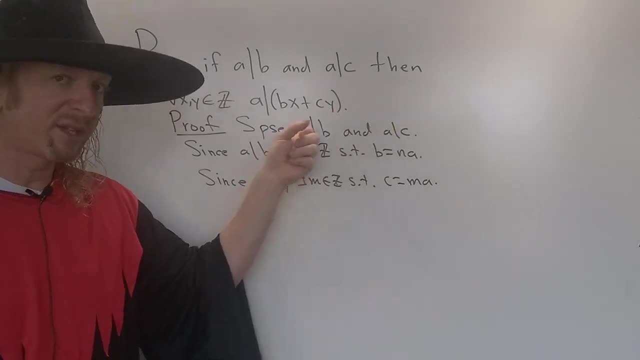 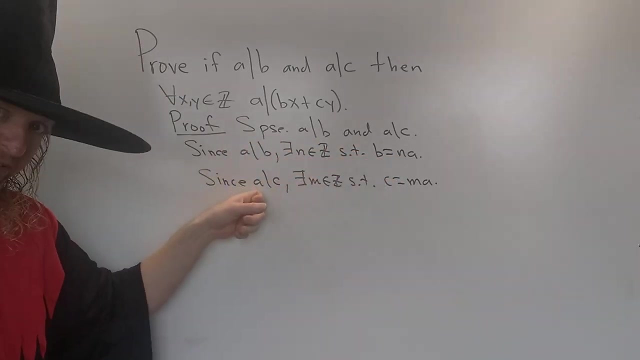 And then I carefully rewrote it again. so I wrote the assumption down together and then I broke up each individual statement. So since a divides b, b is a multiple of a. Since a divides c, c is a multiple of a. 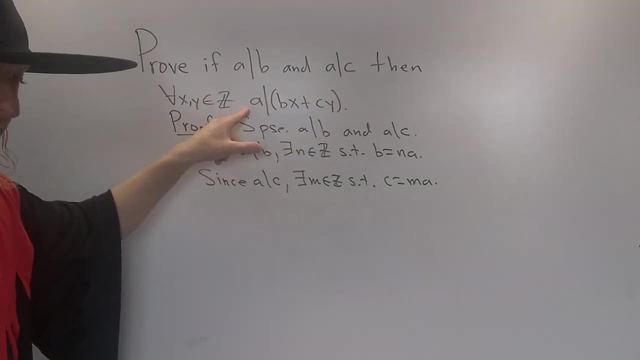 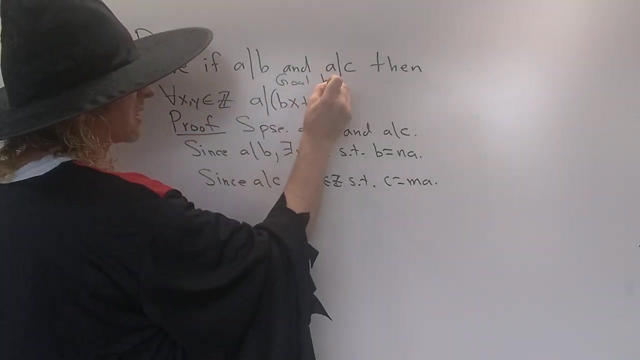 Now we have to show that bx plus cy c is a multiple of a. So our goal right is to show that a divides this, so that means that bx plus cy is equal to an integer times a. That's our goal. That's what we have to get right. 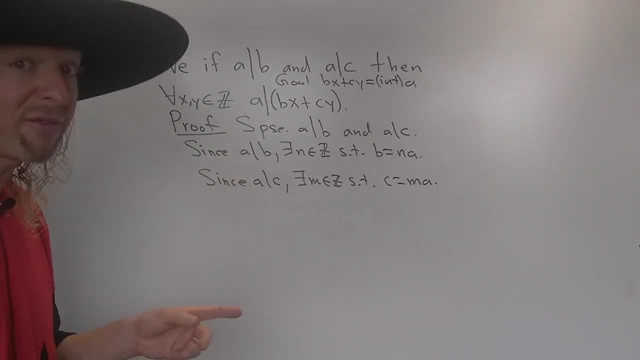 It's really important to know the goal, especially in a problem like this. So I haven't done this problem until like right now. This is my first time doing it. I probably did it a long time ago, a couple years ago or something. 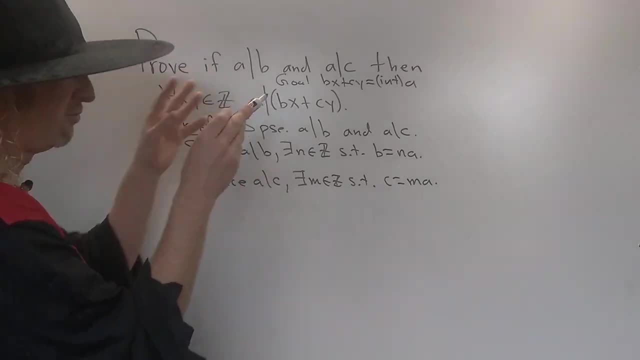 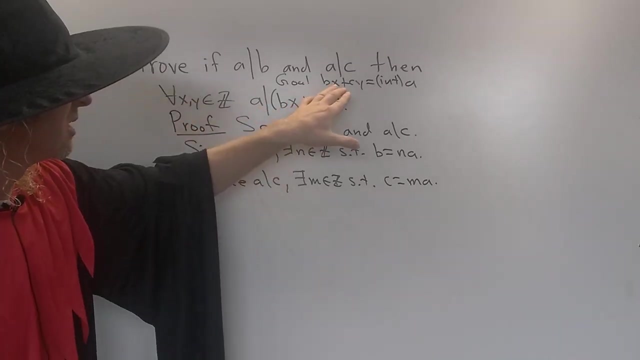 but how am I able to do it again? Because you always have to know where you're going right. So if you write down your goal, you can usually figure it out, like we're doing now. So the goal is this, right. 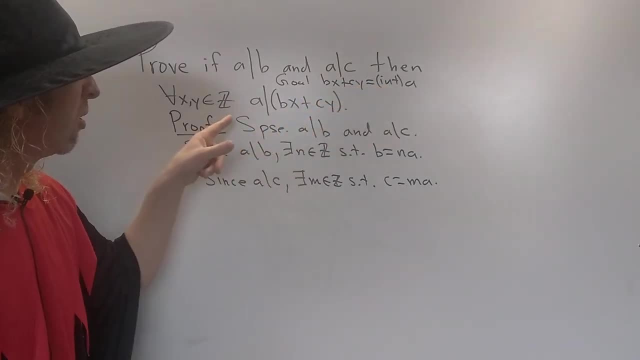 a divides b, so bx plus cy is an integer times a. So this has to be true for all x y. So to properly prove this, we have to say: for all x y. So then for all x y and z. 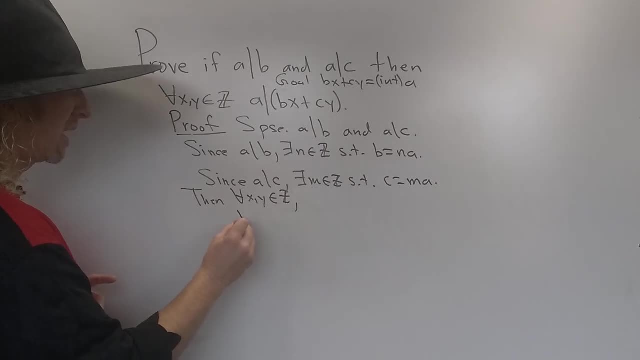 let's look at the quantity bx plus cy. So bx plus cy, This should be an integer times a. So what is b? Well, b is na right, So this is nax right, So this is nax plus. and what is c? 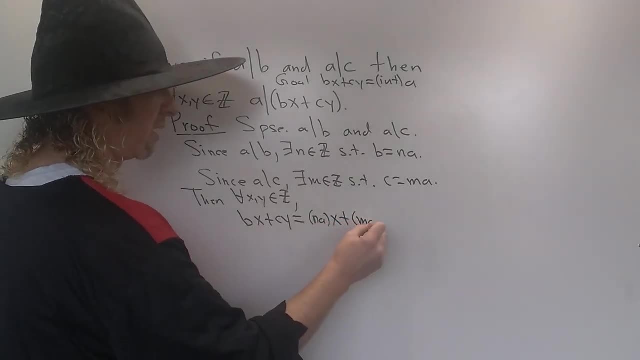 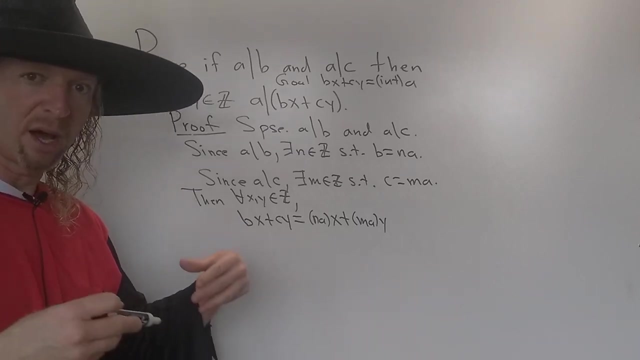 Well, c is na right. So this is, this is nay right. And then we want to write this: we can use some properties here- commutivity, associativity- and you can just pull out the a. 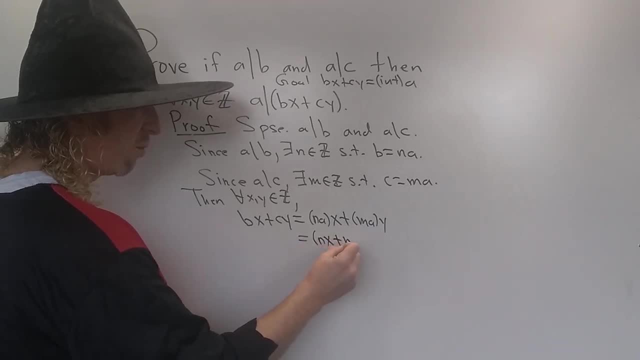 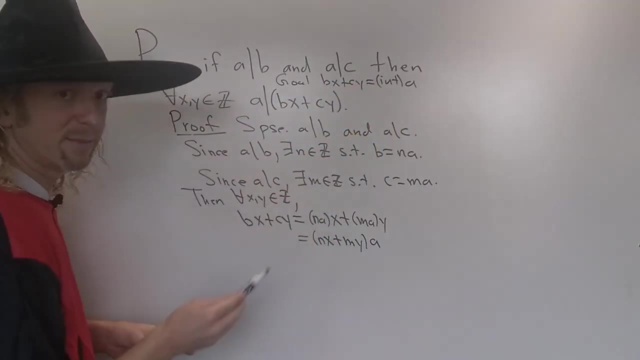 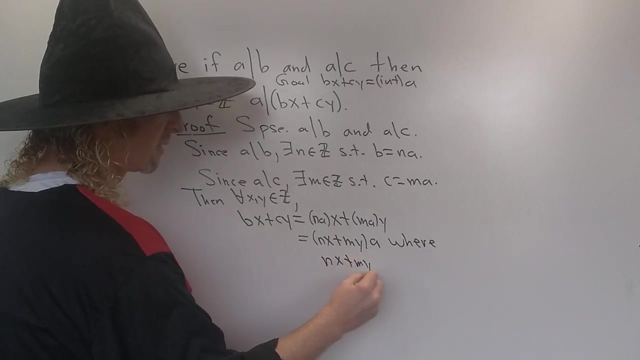 You can write this as nx plus ny and you can pull out the a. So why are we doing that? Well, because we want it to be an integer. we want it to be an integer times a right. So this is an integer, where nx plus my is an integer y.